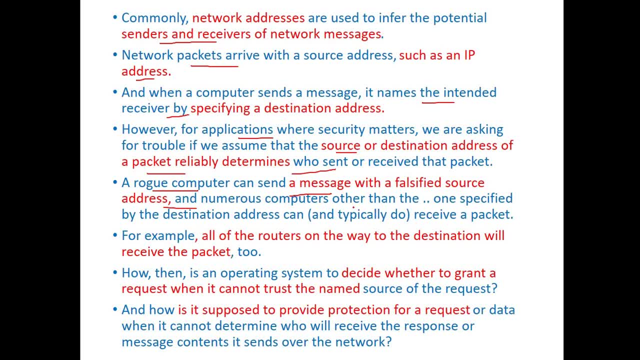 Therefore the message will reach to the computers who is not intended for that particular message, or numerous other computers on the way to reach the destination, Because all the routers on the way to the destination will receive the packet. So therefore it is a problem. 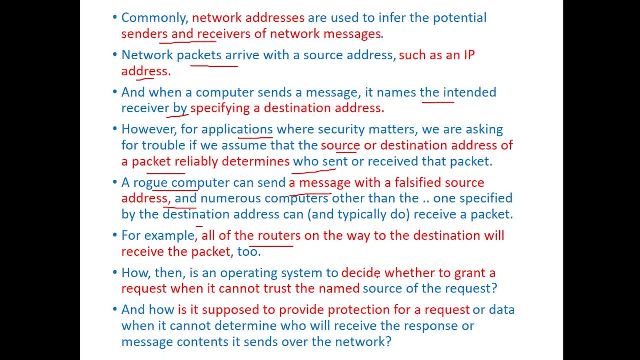 It is an operating system to decide whether to grant a request when it cannot trust the name resource of the request. So that means if the operating system is not able to trust the source of the request, then it can decide whether to send the reply to that message or not. 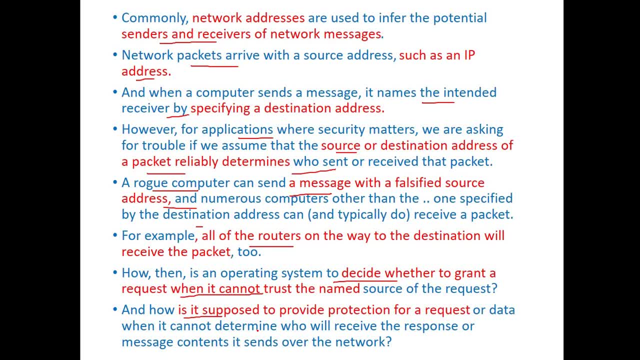 And the operating system is supposed to provide protection for the request or data. When it is not able to do that, it will not be able to send the message. It is not able to determine who will receive the response or message contents it sends over the network. 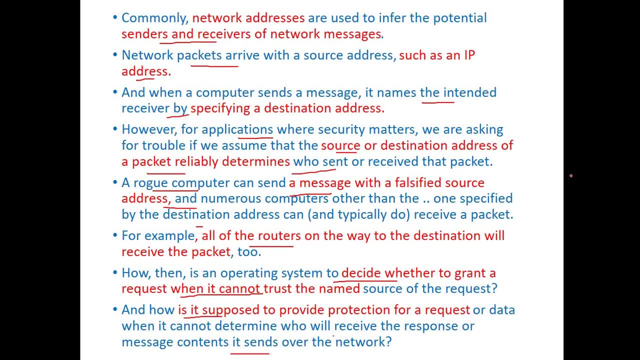 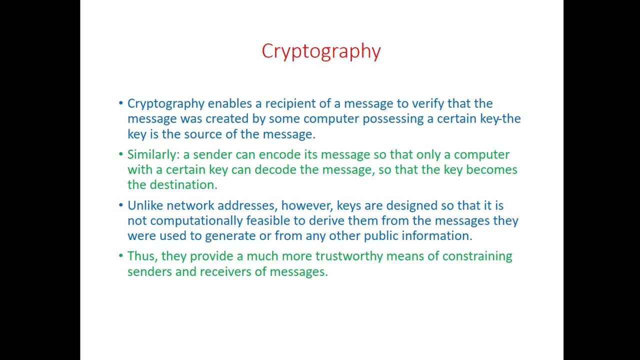 So these are the two responsibilities of the operating system: to decide on whether to send the reply messages or receive the request messages in the network. In order to solve this problem, the cryptography is the one of the ancient technology used in the computer In order to provide the secure way of transferring the messages between two systems or systems connected in the network. 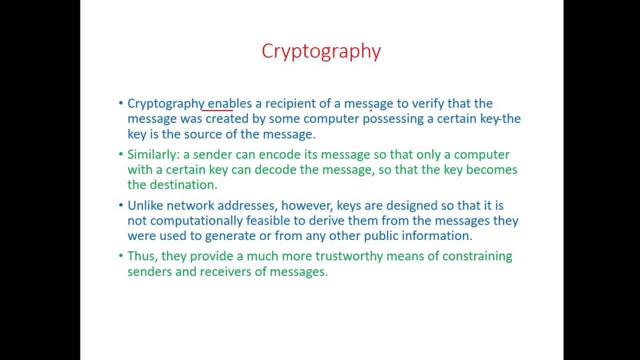 So cryptography enables a recipient of a message to verify that the message was created by some computer possessing a certain key. The key is the source of the message. Similarly, the sender can encode its message So that only the computer with certain key can decode that message. 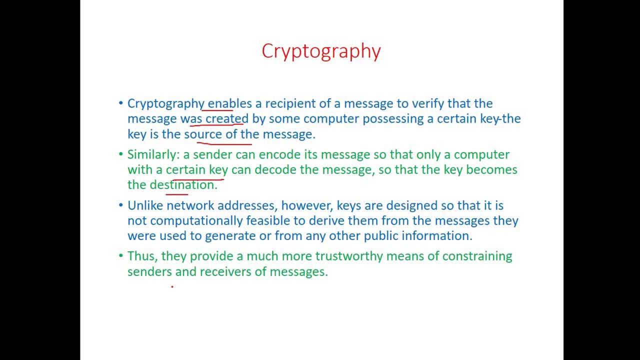 So that the key becomes the destination. Unlike network addresses, the keys are designed in such a way that it is computationally not feasible to derive them from the messages Or not feasible to generate them from any other public information. Thus they provide more trustworthy means of sending and receiving the messages in the network. 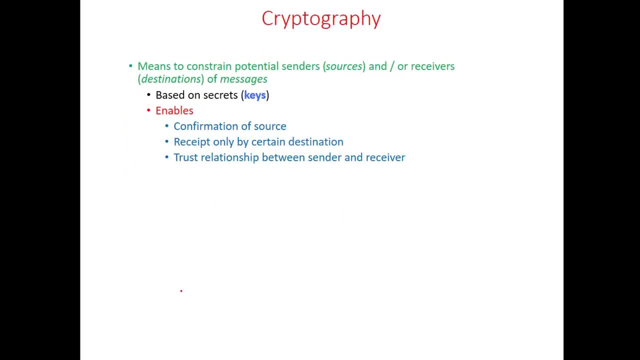 So cryptography means it constrain both senders and receivers of the messages. The cryptography technique is based on the keys. It enables the confirmation of the source. It enables the receipt of the message only by the key And by the certain destination. It establishes the trust relation between the sender and receiver. 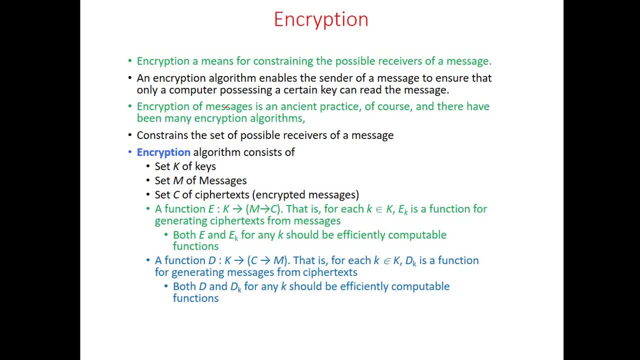 Encryption is a means for constraining the possible receivers of a message. An encryption algorithm enables the sender or receiver of the message to ensure that only computer possessing certain key can only read the message. The encryption of messages is an ancient practice And they have many encryption algorithms. 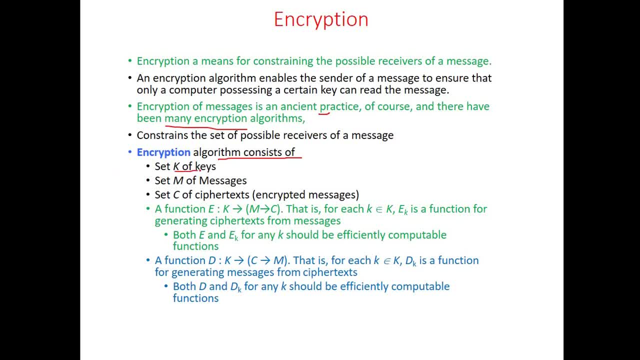 One of the encryption algorithms. here K is set of keys, M is set of messages, C is set of ciphertexts. The encryption function E converts the message M into a ciphertext C by applying the key K. A decryption function D decrypts the ciphertext into letters. 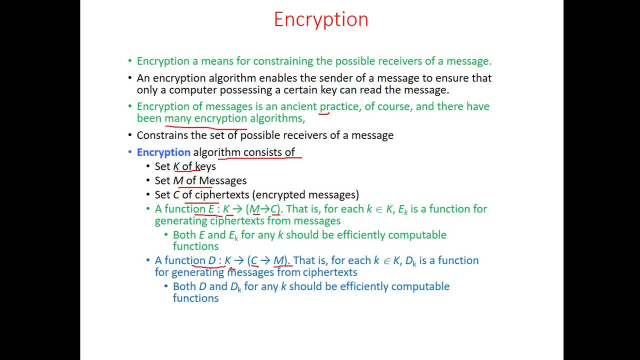 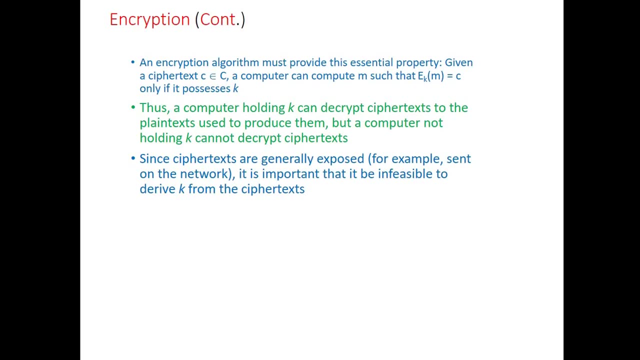 A decryption function. D decrypts the original message by applying the decryption key. So therefore the encryption key E- K and decryption key D- K should be efficiently computable functions. An encryption algorithm must provide this essential property Because, given the ciphertext C, A computer can compute the message M. 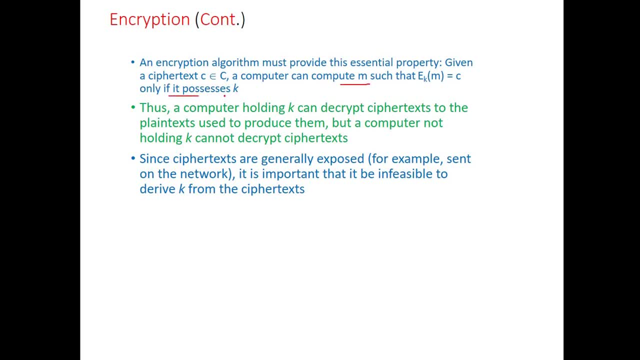 From the ciphertext C, Such that if it possesses the key K, Thus a computer holding K can decrypt the ciphertext to the plaintext, But a computer not holding K cannot decrypt the ciphertext. Since ciphertexts are generally exposed, It is very important that it is infeasible to derive K from the ciphertext. 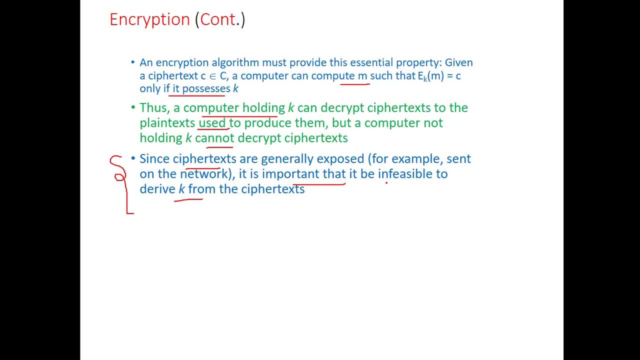 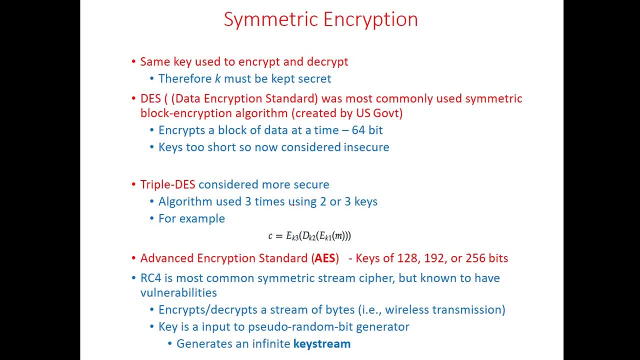 It is very important that there should not be any possibility to derive K from the ciphertext. Symmetric encryption uses same key for encryption as well as decryption. DES is a data encryption standard. It is one algorithm that is most commonly used- symmetric block encryption algorithm. 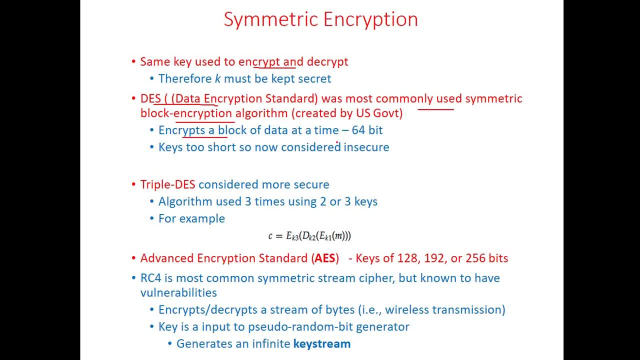 This algorithm encrypts a block of data at a time And the block size of this encryption algorithm is 64 bit. This 64 bit encryption algorithm nowadays is assumed to be too short And insecure nowadays. So, therefore, and another variation of the DES algorithm. 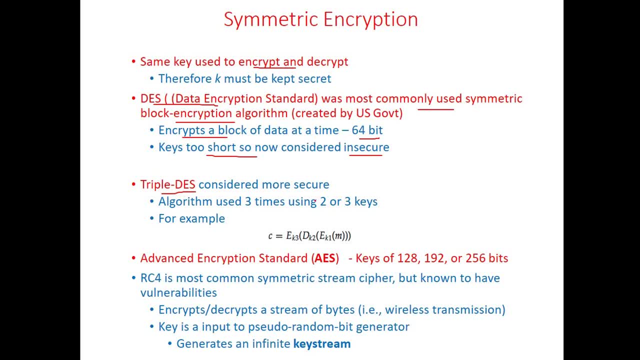 That is, triple DES algorithm is used. It is considered as a more secure algorithm Because it uses Three times the DES algorithm, Using two or three keys, For example. First, the message is encrypted by using first key K1. And whatever message is, whatever ciphertext is obtained. 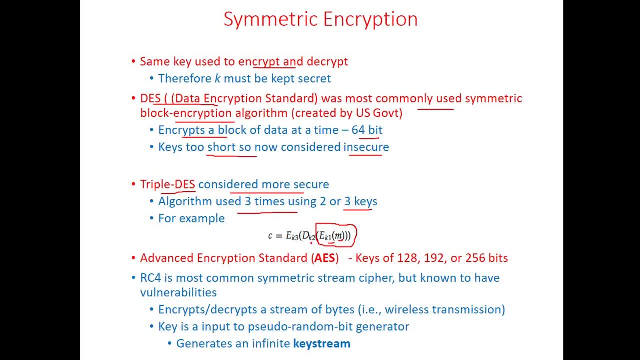 It is decrypted with K2. And whatever output is obtained from this application of K2. That message will be again encrypted with the help of the third key. So that means the output of the first key is input to the encryption function With key K2.. 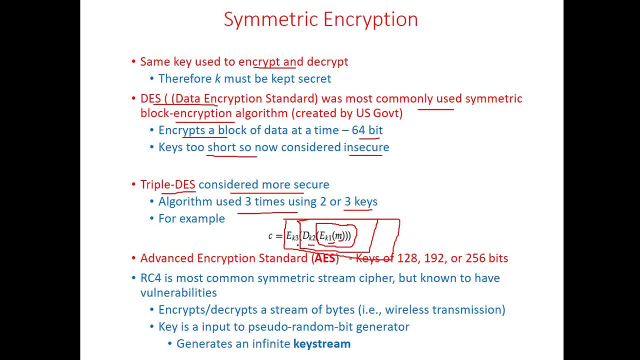 Then the output of the encryption function with K2. Will be an input for the encryption function K3. So likewise, three times this DES algorithm is applied. Finally, whatever output is generated, That is treated as the ciphertext And is transmitted over the network. 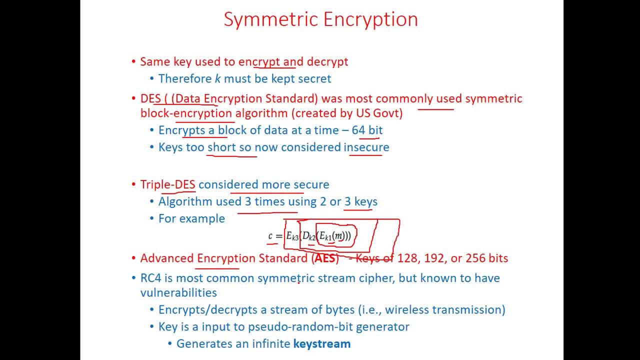 Advanced encryption standard, AES is the another encryption algorithm. It uses 128 bits or 192 bits or 256 bits of. It encrypts a block of size- Either 128 bits or 192 bits or 256 bits. So RC4 is another most popularly used encryption algorithm. 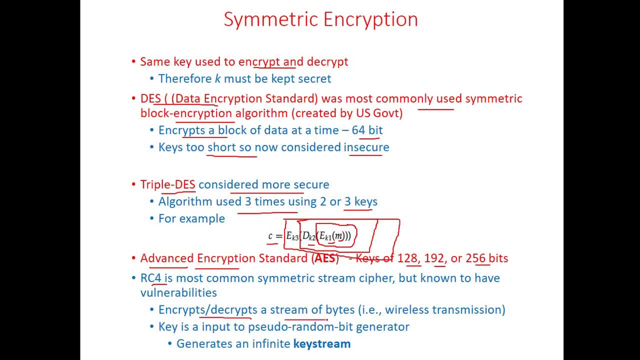 It uses the encryption or description For a stream of bytes. That means it will apply this algorithm For a stream of bytes, Byte by byte, it will encrypt or decrypt, So like that it generates an infinite key streams. Let us take up an example. 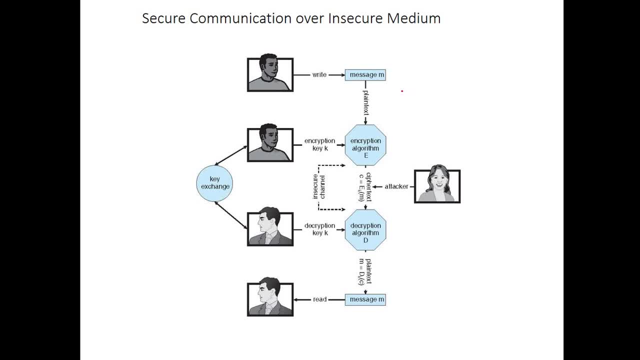 How this symmetric encryption Performs. Initially, The message M Is written. This message M is considered as a plain text. It is Applied to the encryption algorithm E. The user Encrypts the Given plain text By using the encryption key. 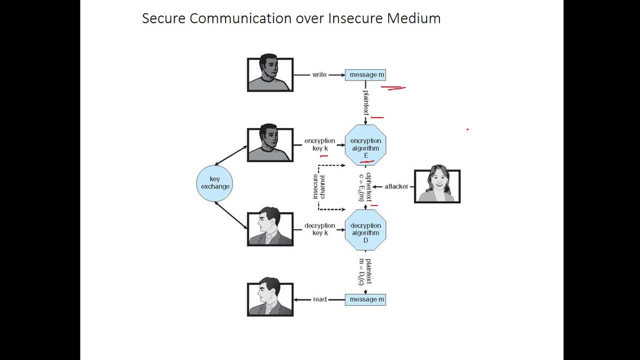 K. It is a type Cybertext C. C is the cybertext generated By applying the Encrypted Key. So In the network, If an attacker is trying to Find the message in the network, The attacker could see only. 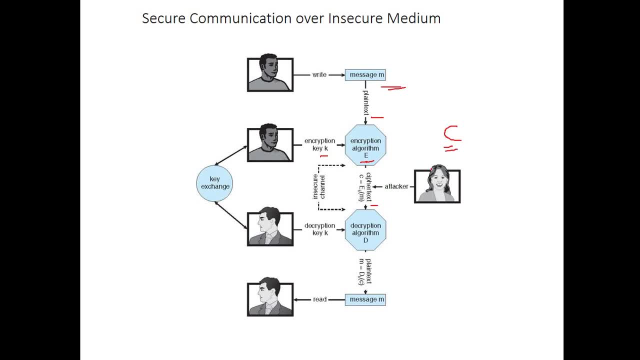 The encrypted form of the message, That is, Cybertext C, So therefore The attacker could not Interpret What the message is Originally. Then The cybertext will be decrypted At the Receiver side By supplying a. 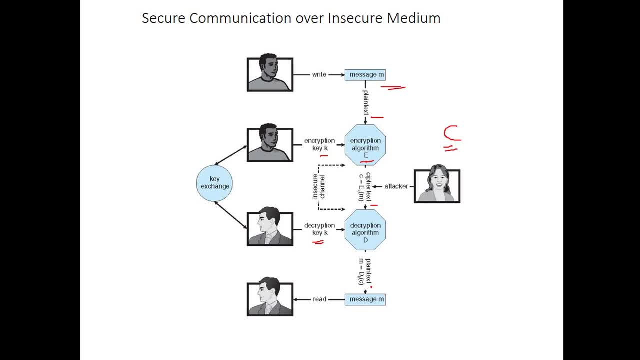 Decryption Key K. A plain text is generated Once the decryption is done With the Decryption Key And finally, That message will be Read by the Receiver. So this is the Secure Way of. 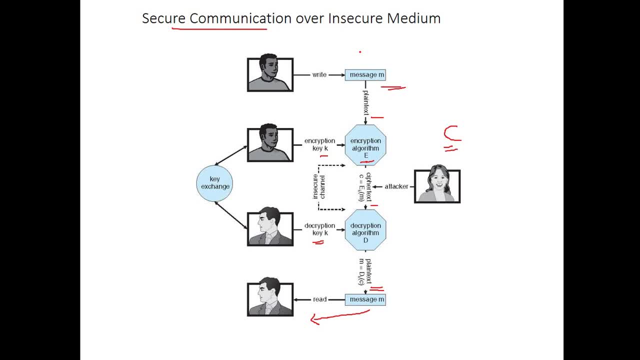 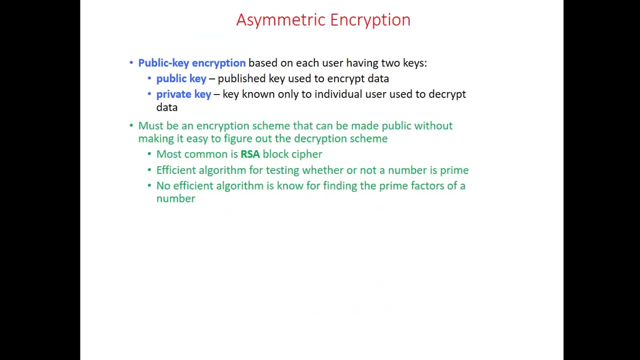 Communicating Over the Insecure Medium With the Help of The Symmetric Encryption. Here, The Key Used For Both Encryption And Decryption Is Same. That is Why. 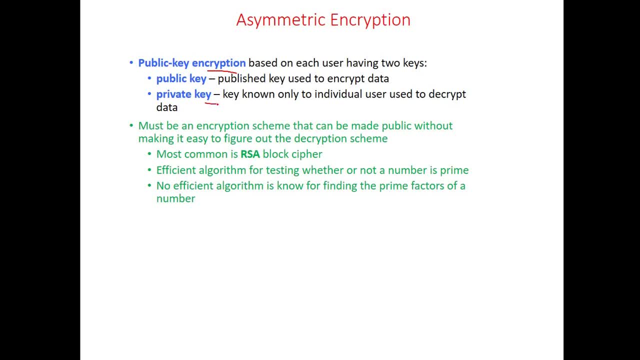 It Is Called As Symmetric Encryption. Here The Key Used For Encryption, Which Is Used For Decrypting The Cybertext, Is Called As Private Key. 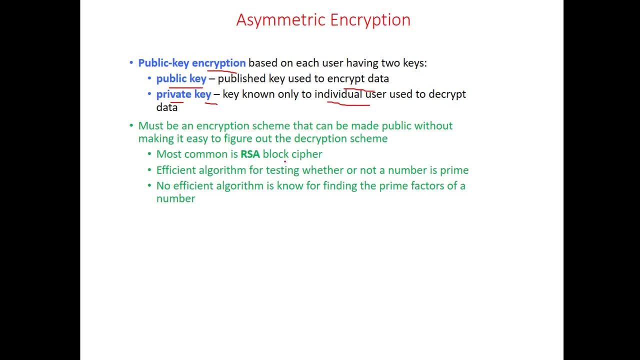 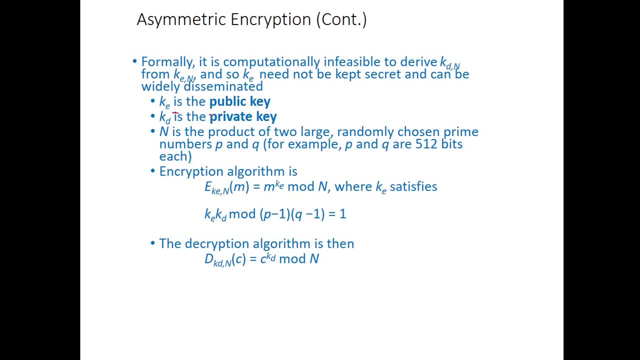 This Encryption Key Is Made Public Because It Is Not Possible To Find The Private Key From Each Prime Numbers P And Q. The Message M. 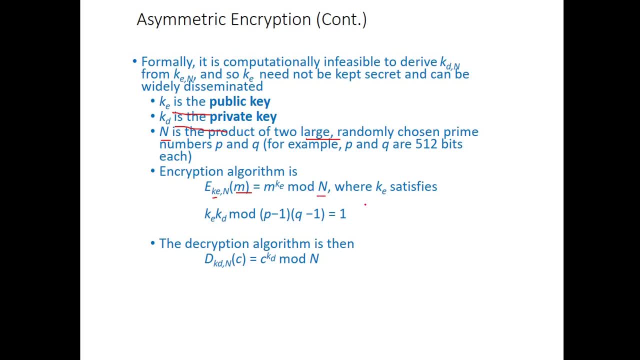 Is Encrypted With The Help Of This Encryption Key K E And The Number N. The Decryption Key K D Is Made With Encryption Key. 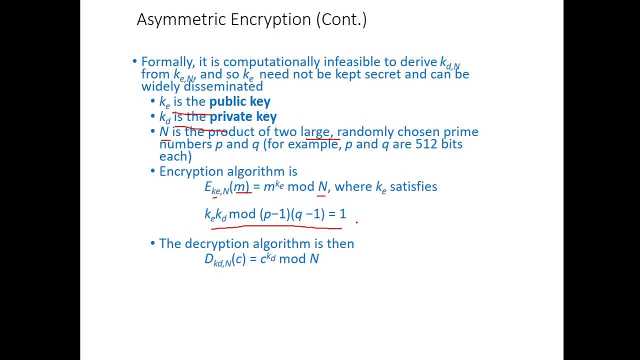 This Product Mod. The Product Of P Minus One And Q Minus One Is Equal To One. This Condition Satisfies For The Encryption Key. 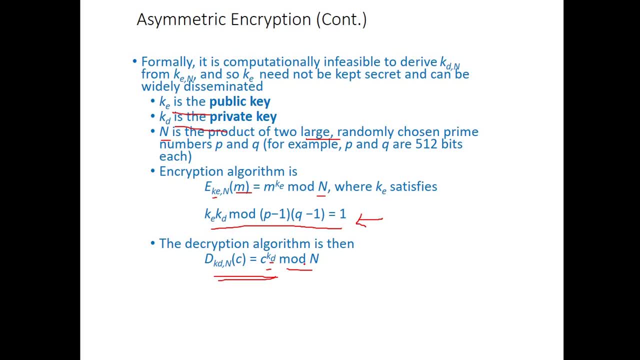 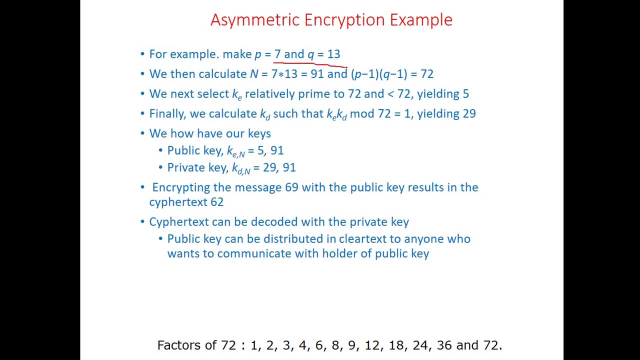 And Decryption, And It's A Decrypted Message. Let Us Take Up One Example For The Asymmetric Encryption. Let Us Consider Two Prime Numbers: P. 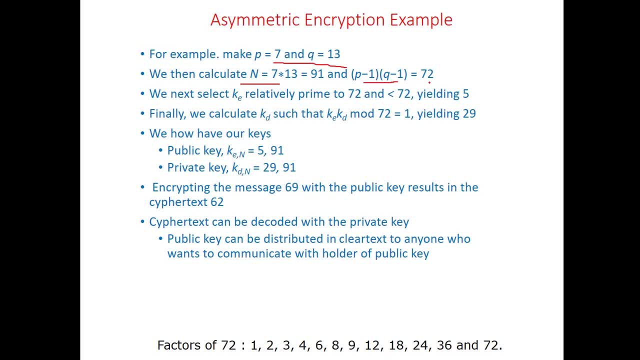 And Q. The P Is Equal To The Encryption Key. K. E Is To Be Chosen, Which Is Relatively Prime To Seventy Two Here. 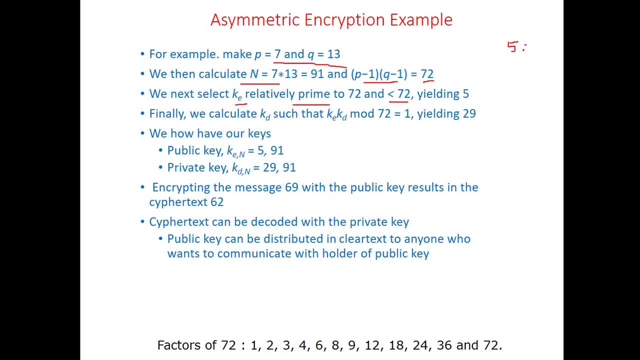 A Relatively Prime To Seventy Two, And It Should Be Less Than Four, Six, Eight, Ten, Like This, Up To Seventy Two. These Are. 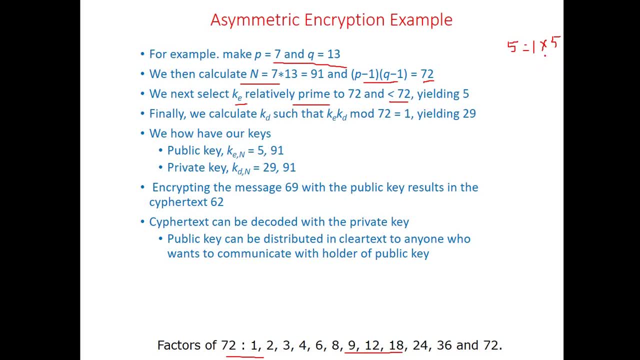 The Factors Of Seventy Two, So Five Is A Relative Prime To Seventy Two Because, Other Than The Decryption Key K D From This. 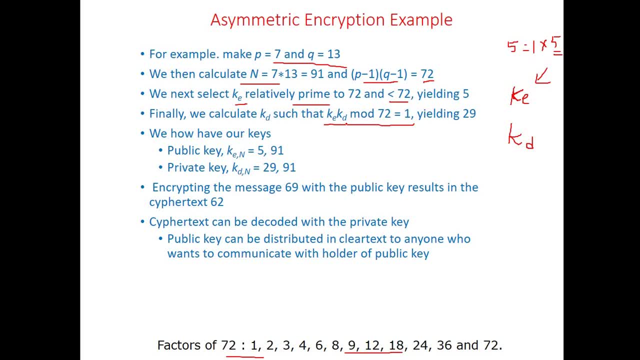 The Equation To Be Satisfied Is: K E, K D: The Multiplication Of K E And K D Mod P Minus One K D. 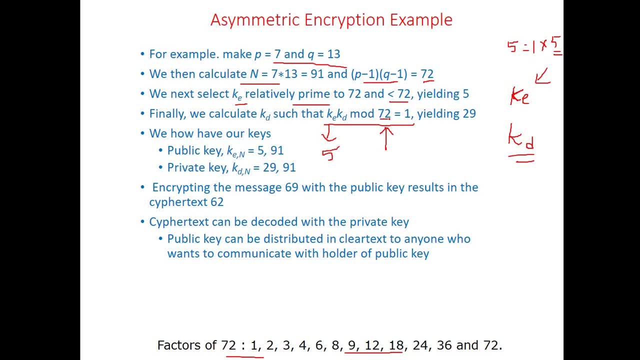 Is Substituted As Five, And We Know The Value Of P Minus One And Q Minus One, That Is Seventy Two. So This: 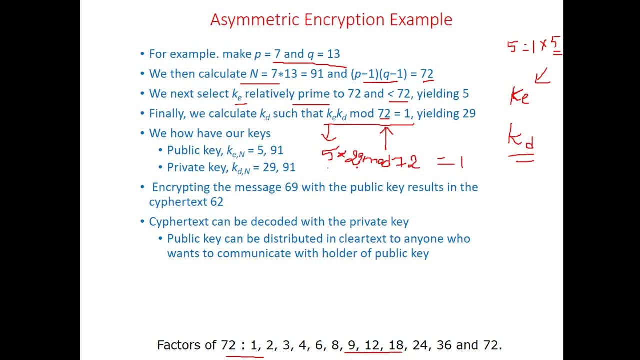 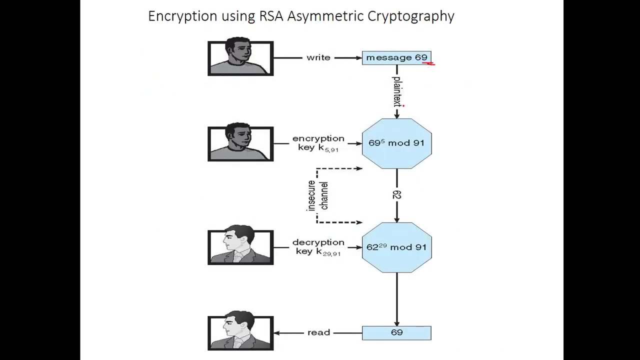 Should Be Equal To Satisfied. If We Take The Value Of K D As Twenty Nine, So Twenty Nine Will Become K D Decryption Key. 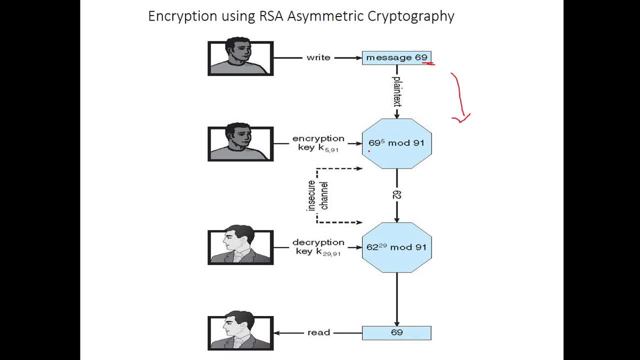 So Now We Want To Encrypt The Message. Is The: Given The Message: M Power: Apply The Encryption. Key K E Mod: Apply The Mod Function. 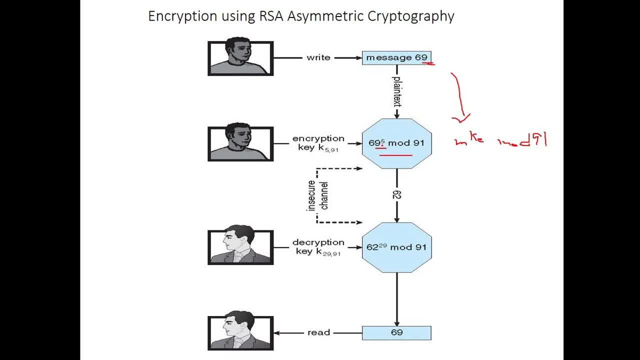 With Ninety One. So This Sixty Nine Is The Original Message, Which Is Cyber, Cyber Text. This Cyber Text Is The Encrypted Version Of 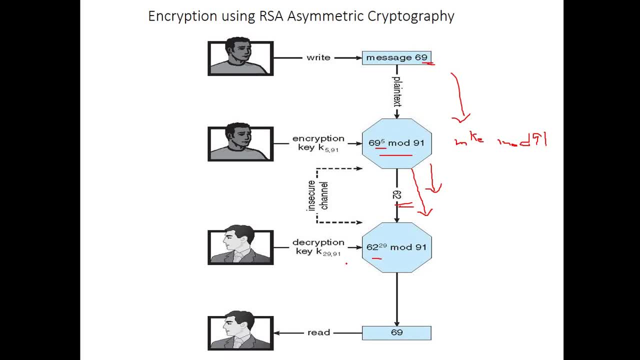 The Plain Text. This Cyber Text Will Be Transmitted To The Destination Over This Insecure Channel. Once This Will Be Transmitted To The Original. 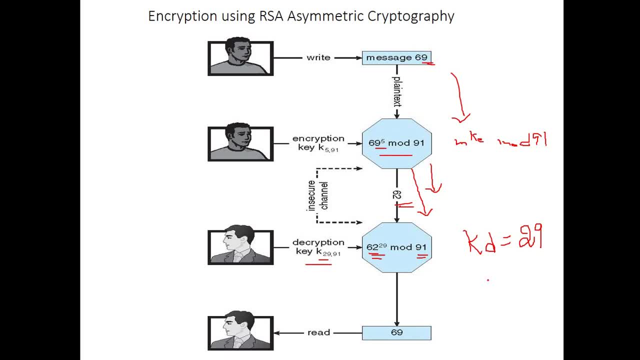 Text Back. That Is Sixty Nine. So Sixty Two Is Raised With The Power Of Twenty Nine, And Mod Ninety One Is Applied, Cyber.